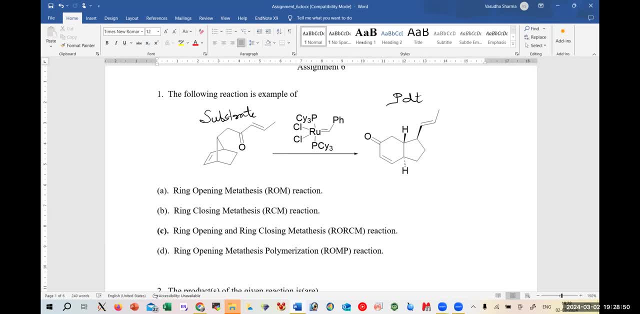 is named as what Is it ring opening metathesis? Is it ring closing metathesis? Is it ring opening, ring closing? or it is ring opening metathesis- polymerization- Okay, we know that this seven member ring has been called as a polymerization, So this is a polymerization. 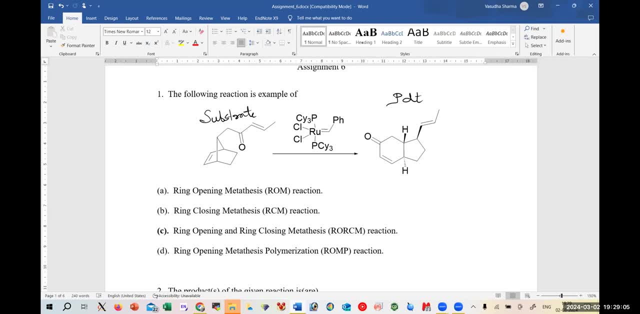 and the six member ring has been opened to form this six member during. for sure, it's a ring opening, but also there has been some ring closing also. That's why we could see that five member thing is here and then yeah, and to see is correct, because we just have. 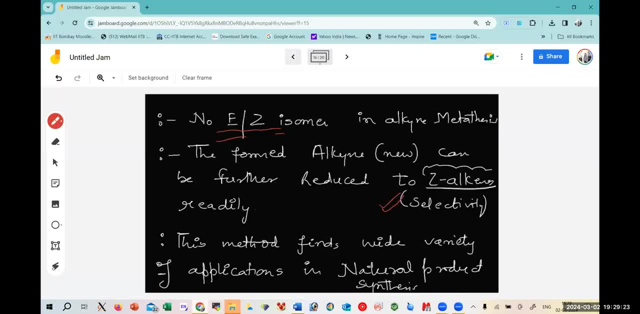 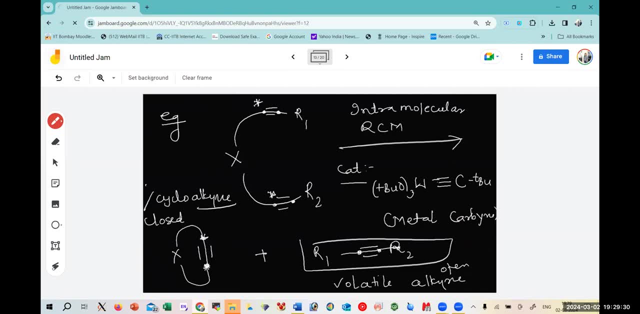 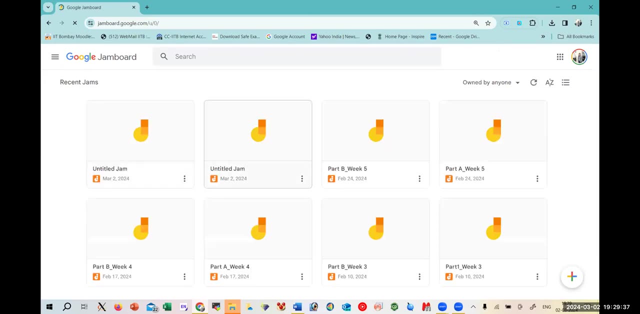 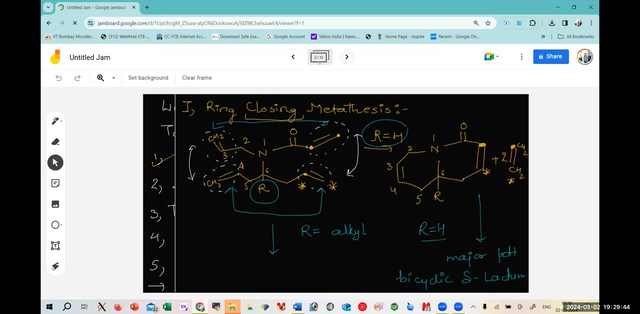 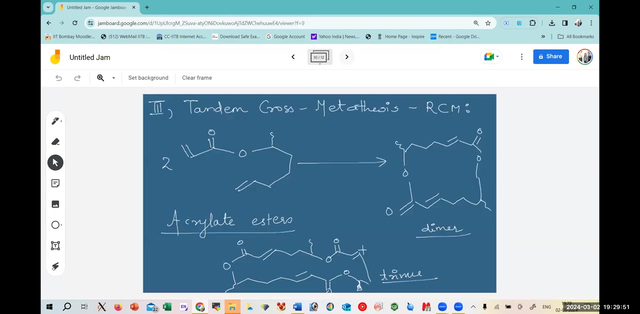 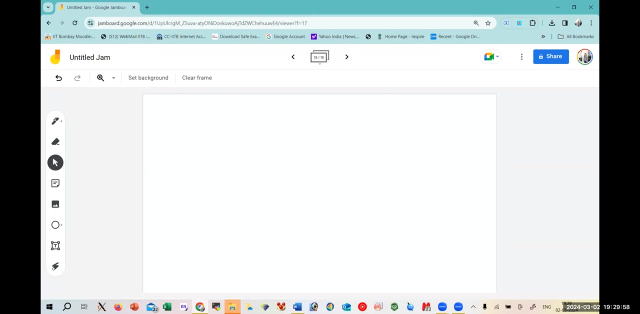 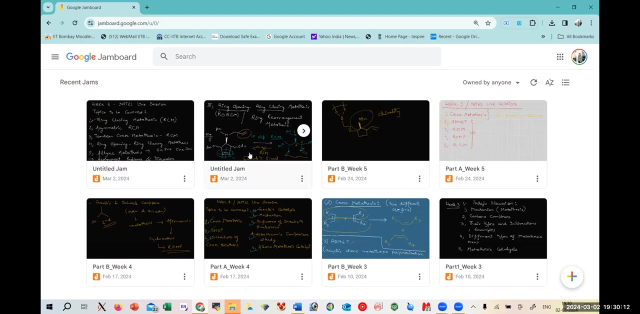 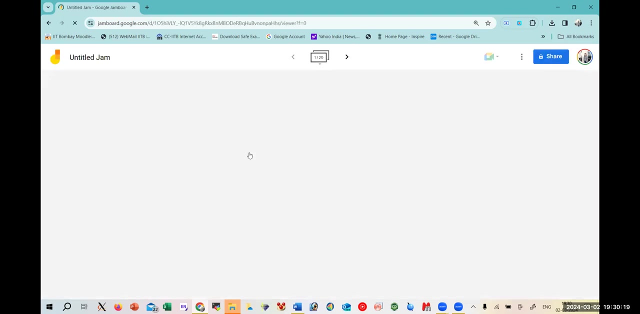 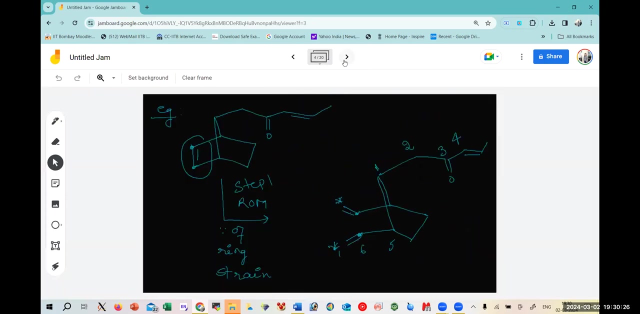 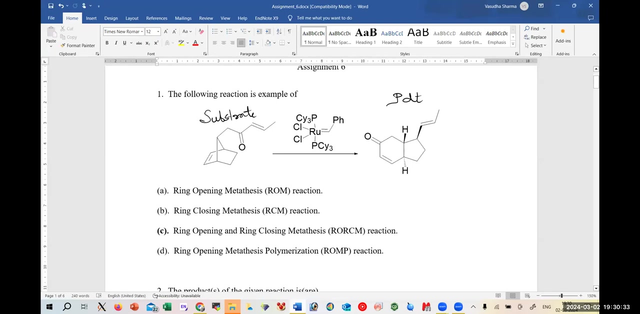 seen this example. If I just open the ring, opening just a second, I'll show you the you. yes, we have taken this example, so here this one. so the way we have taken this example- yeah, it's the exactly same example. we have already explained that. firstly, this particular 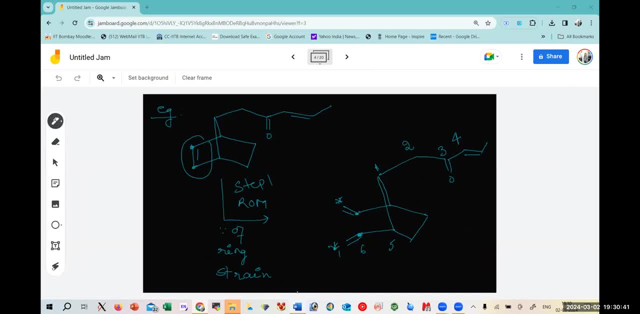 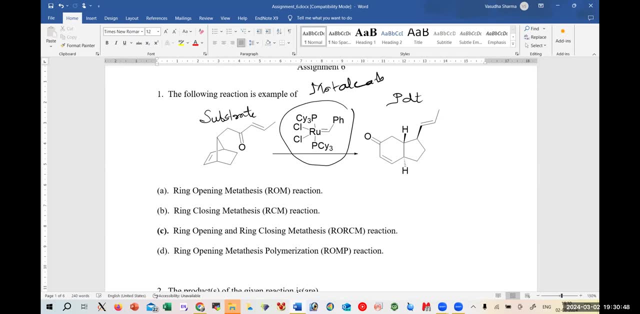 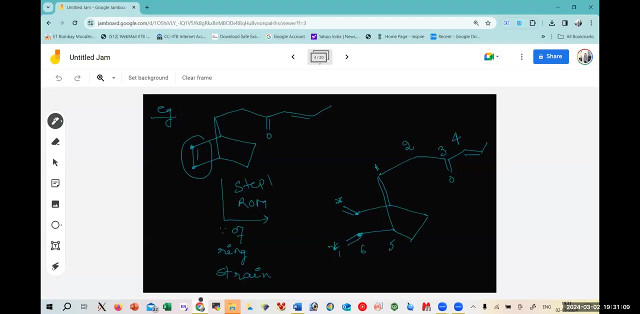 because the catalyst that has been used, this is your metal carbene catalyst and it is nothing but the first generation catalyst. and in presence of this, it is undergoing ring opening of the strained norborene bonene system. and then that would combine with your L key. firstly, it will open. 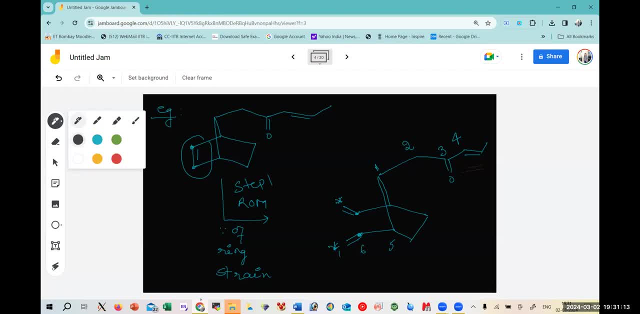 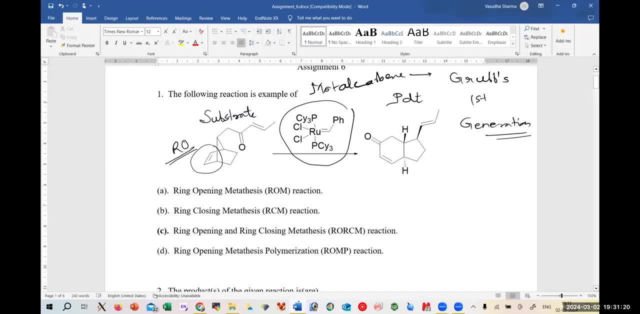 and this will then combine with this particular L key to give you the desired product, which we have already seen, and it would give you a six membered and five membered ring where it has not asked for the product- which product has already been given, but the answer is your. 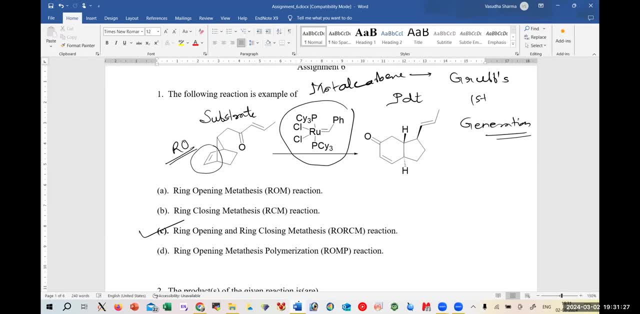 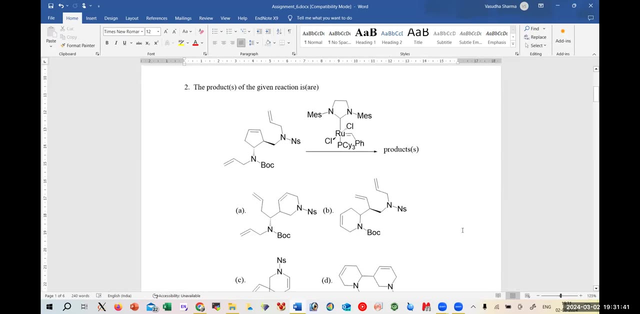 ring opening and ring closing metathesis reaction. so if the answer was right, which you have given, we can go to your next example. okay, so here we have another example where, again, if you will see, it's another type of grubs catalyst, it's a second generation, these kind of grubs catalyst has also been explained. 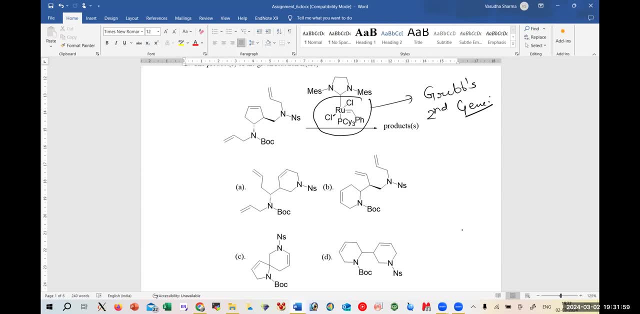 already in the previous lectures. if you have missed the sessions, then please go back and check them. okay now, if you will see it carefully, we have one L key over here, another L key over here and one L key over here also, which is a closed one. so, firstly, when we have seen, 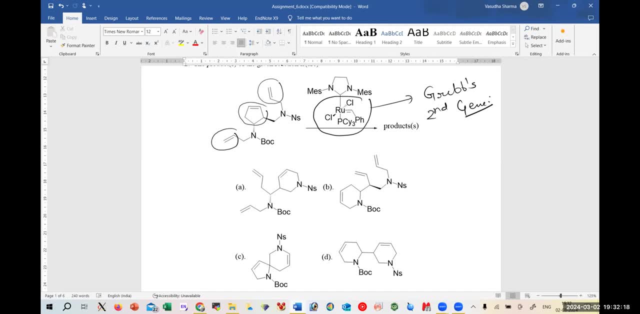 that how the reactions undergo when we are having a grubs second generation. so firstly it will undergo the ring opening and after the ring opening thing it will undergo the ring closing mechanism. but it would happen in the second generation. so this is the second generation. Here you can see that in the second generation. so was there golden R, a number I have referred. 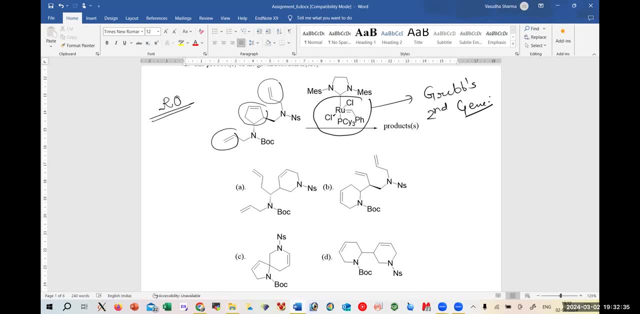 to a plate surface is. must I show you a 보면? I have shown in here. we have noticed this empty, but made more visible. toi, here is the idea that it's possible to see the 11th, the e group, but you can also see that in the second generation, which was preceded by the second generation, a little more visible. 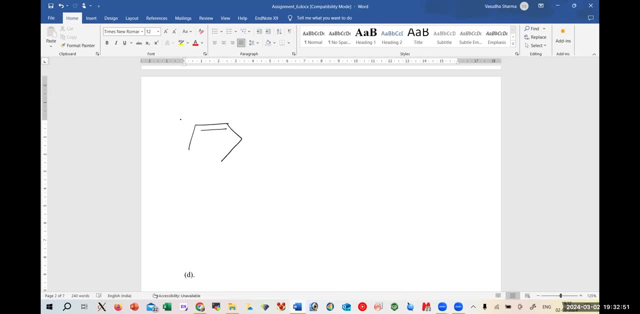 and on the upper left, how here after this machine, I am finding the same reaction in here, because once again this is the same reaction in here삼. also here I am Pobs here, far match it even just you can see that Jess n in you become. able to see that again at the不同 area here. Don't miss the place means please try to do it on your own. so please, don'tuggling. so for you still re. if you are really liebered that paper, you want some time to re-examine your. 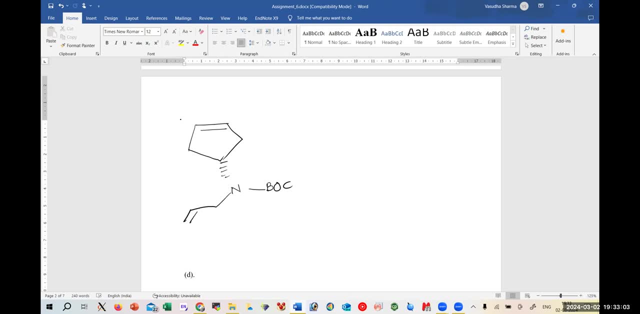 and one alkene group here, and the other part is N and this is some other group, NS. so now, firstly, it will undergo ring opening, and ring opening could only be formed if these twos are having alkenes over here. so it would be like this way: 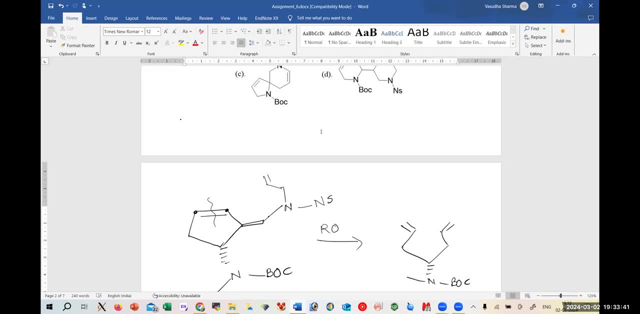 and Bob, and here it is, having oxygen elements. we have done ring opening part. now we have different choices: to combine this thing or to combine this thing to give us the product. so what will happen, what whichever, the rings very close because these two can't combine with each. 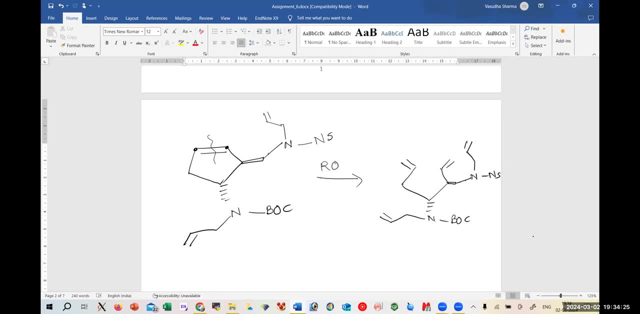 other. we have already opened it. it's a strain one you can just check. this is one part of the ring opening part. now we have 2,, 3,, 4,, 5 and 6.. This will make a 6-membered ring: Now 1,, 2,, 3,, 4,, 5 and 6.. I'll just mark. 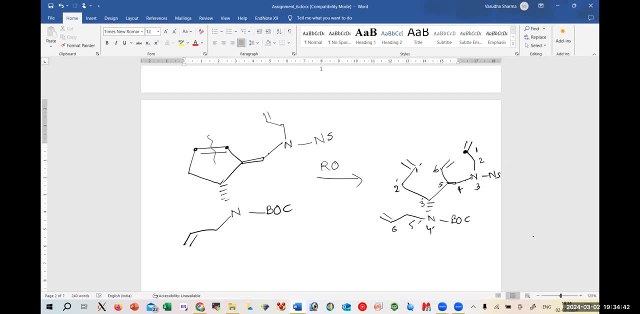 it as dash 3, dash, 4, dash 5, dash 6, dash. So this side also, it will give you a 6-membered ring. So when you have a 6-membered ring option comparative to the 5-membered ring always. 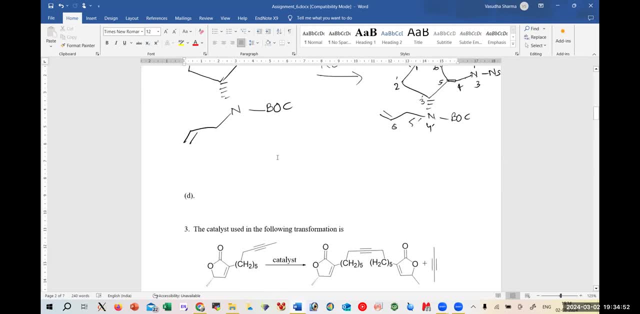 it will go for the most stable ring. So what it will form. So then it would ultimately be forming a 6-membered ring, which is: we'll just take two 6-membered rings, and in the two 6-membered rings, if you'll just carefully see, there is a carbon-carbon bond. So we will. 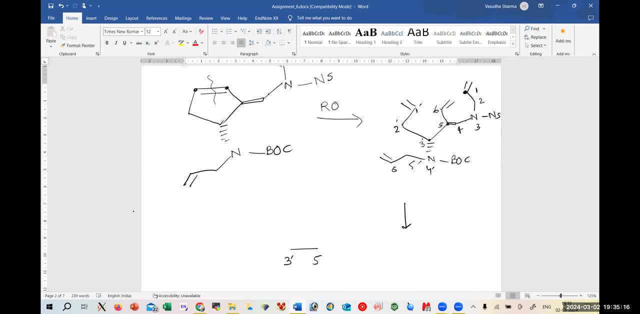 just make a carbon-carbon bond which is 3 dash and 5 dash, 5.. Now this 5 is related to the 6, which is combined with 1, then 2, then 3 is nitrogen, which is having an S group. 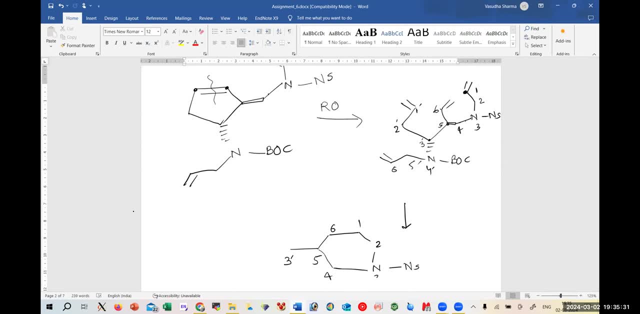 5 is combined with 4, and this is combined with nitrogen 3.. Now 1 and 6 was about to have the LTE. Similarly, other hand go to 2 dash, then 1 dash. 1 dash is going to combine. 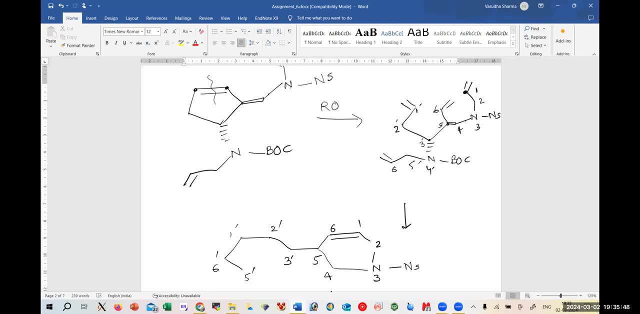 with your 6 dash, then 5 dash, 6 dash, 5 dash, 6 dash, 7 dash, 8 dash, 9 dash, 10 dash, 11 dash, Then 4 dash is your nitrogen. this is your 4 dash and this is your combination. 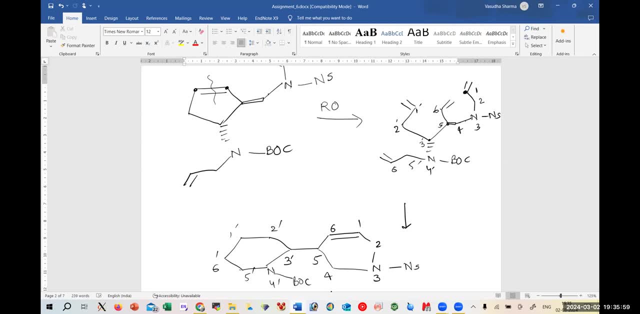 of the nitrogen and this is having a bog group And if you'll see, 1 dash and 6 dash is going to have the LTE, so it is your group. Now, if I'll make it even more properly, so this group is nothing but your. 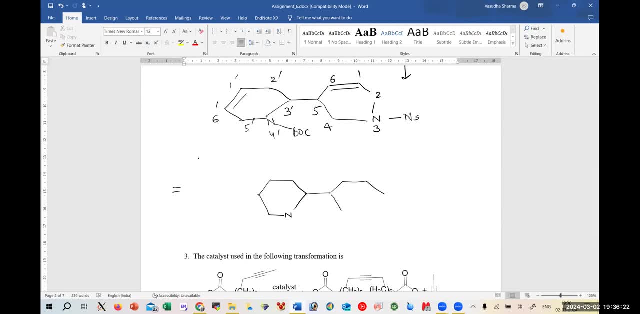 Nitrogen, nitrogen double bond 4,. this is bog and that is MS. So you can easily see that which product that we have formed, and this is matching with our only option, number D. Is this clear? If you have any doubts, please let me know, or else we can move further. Okay, great, So. 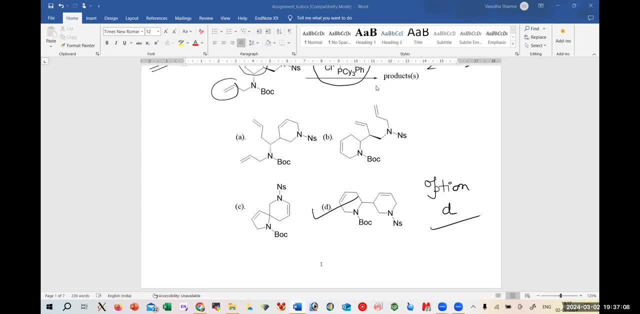 this way only don't get worried just by looking at the substrates- different LTEs- You just have to try out the possible combinations, Best way to give a numbering, and when you have given the numbering, you will get a numbering Okay. so now let's go to our next step. If you have any doubt, please let me know, or else. 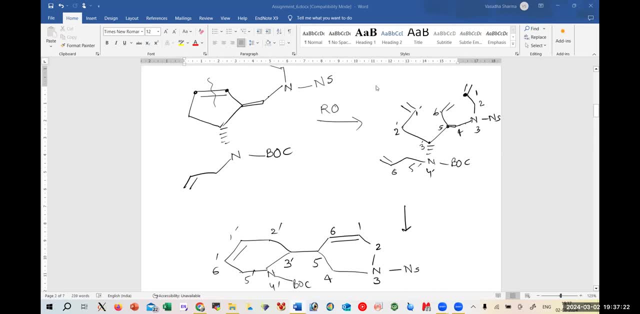 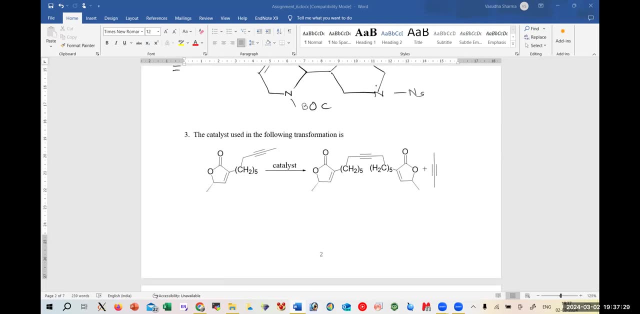 be easily able to find out which kind of products without making any mistake. You can just find out the product. Now let's try this one: The catalyst used in the following transformation. So, if you will see carefully, we have an alkene, but this alkene is still bound. here We have 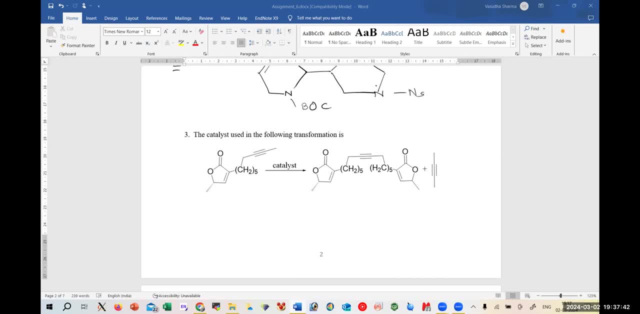 an alkyne and the alkyne is connected to make another alkyne and giving another alkyne. This is your cycloalkyne product, Not cycloalkyne. sorry, It's a new alkyne over here, So first, 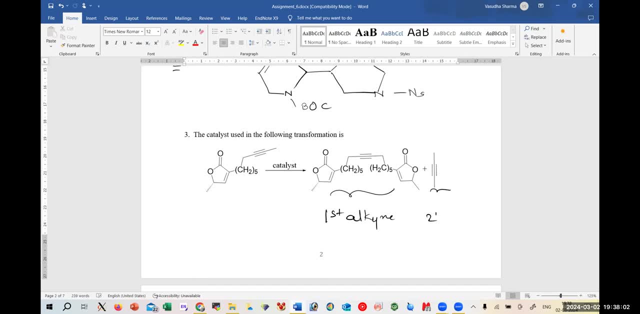 alkyne, which is also open, and this is your second alkyne. So this can only be happening when you are taking two units of this particular group and they combine together to give you another alkyne and the side product of this alkyne. 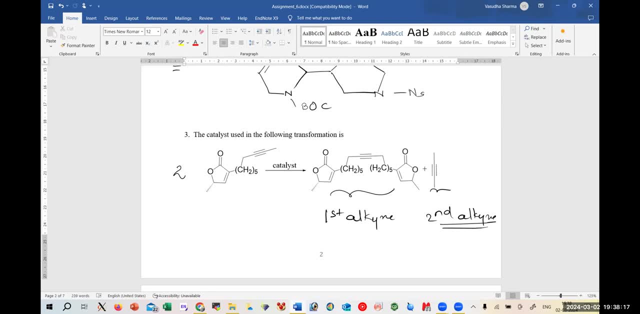 We have done this- I've already seen this example- that I'm just considering this whole group as R. So if R is here, the other part is CH3.. Another R I'm taking, which is CH3.. Now this sorry. 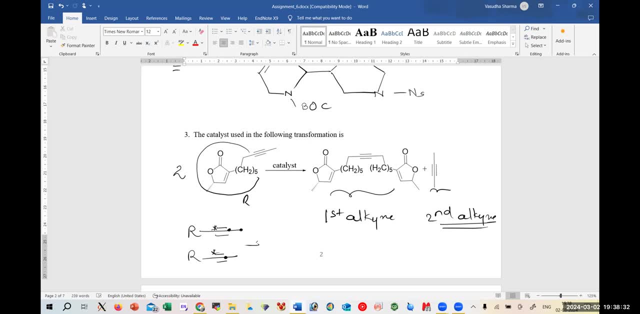 this and this would combine and this and this would combine. So R star triple bond, star R plus dotted triple bond, This dot. So now, if I consider this whole group as R, so this is nothing but my this group and this C and CH3.. This is my this group. So here it is nothing but a self-metathesis. 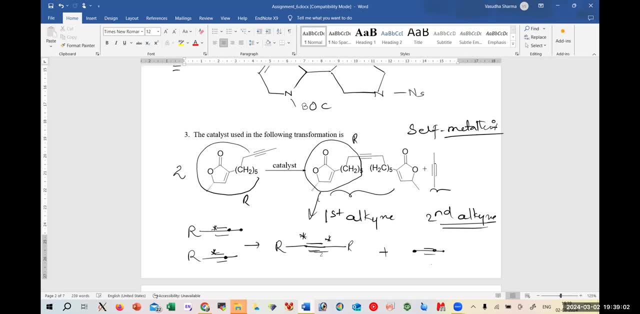 alkyne metathesis reaction is happening in presence of the catalyst. So what is the question? They're not asking for which type of reaction. you should be knowing in and out of the reaction. completely The question could be made from this particular. 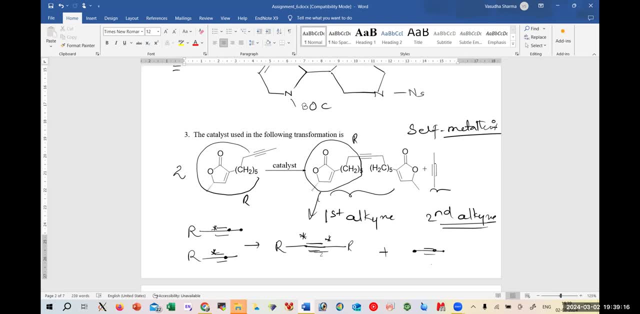 Okay, Part number of questions could be made. They could ask for what kind of metathesis is being happening, as they have asked for what kind of catalyst is being used. So this kind of metathesis where two alkynes are combining together. 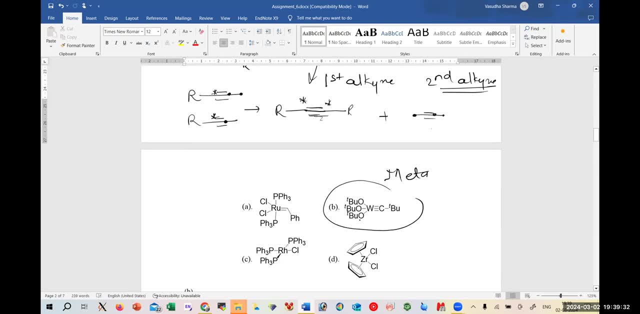 We know that happens in presence of metal carbine. We have seen this is your graph's catalyst that could give that only gives you the alkyne metathesis. Metal carbine is the one which would tend to give you, Which would tend to have this kind of self-metathesis or cross-metathesis of alkyne. The other ones, 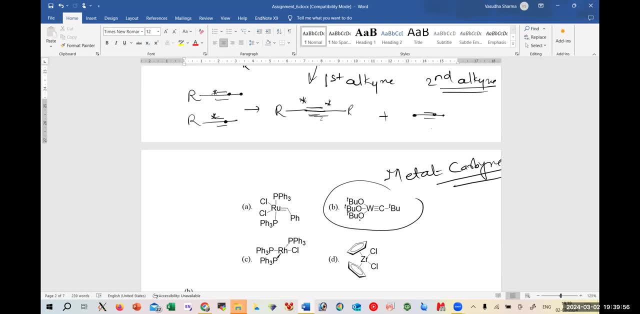 are not the catalyst which are being used for the metal carbine, because metathesis reactions can only be possible when we are having metal carbines or metal carbines, So these could only be possible and these are neither the carbines nor the carbines. 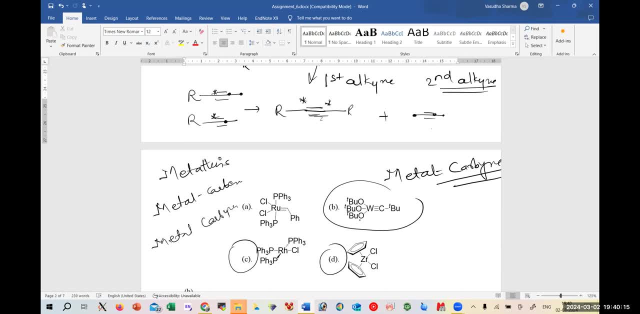 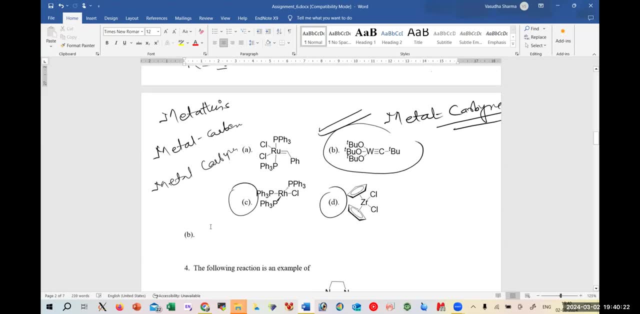 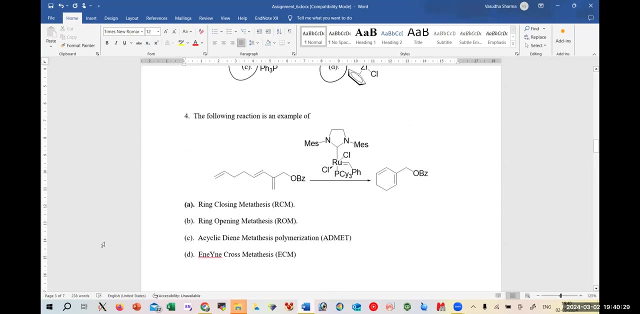 So these are in any way eliminated. This option is only for the alkyne metathesis and the right option is your D. I hope this is clear. Now, moving to our question number four. Okay, The question number four says that we have this alkyne system and this graph's catalyst. 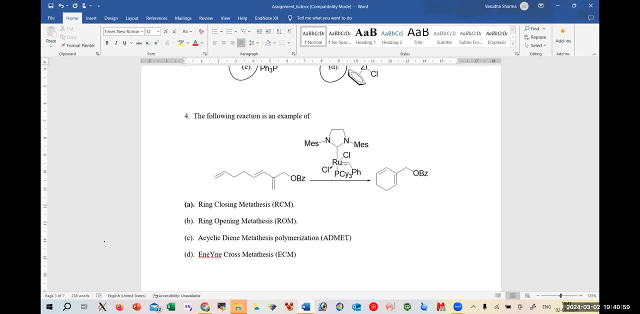 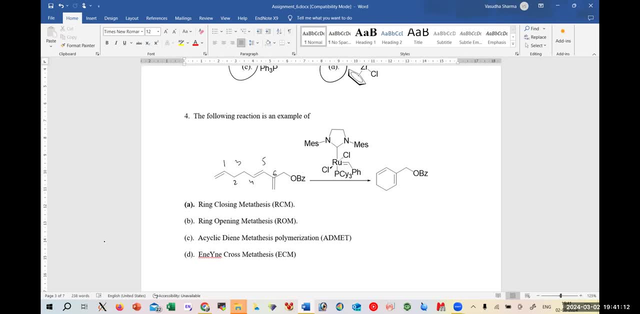 And this is giving you, This one is your, this is 6, this is 1,, 2,, 3,, 4 and 5, and this is your ring closing metathesis. It's very straightforward. Then the substrate of the falling reaction is RR. 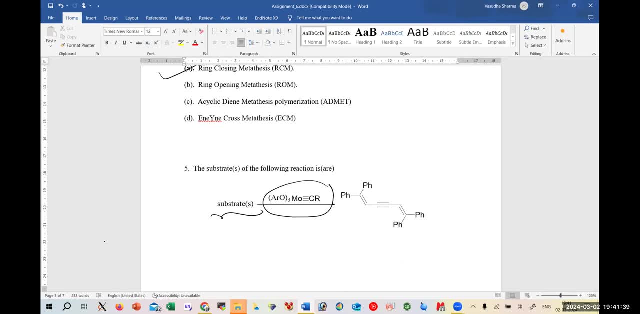 We have the substrate and the alkyne. Now, what would be the substrate which is going to undergo having this reaction? We could only be seeing that this part would be having your different alkynes which are combining together to give you. So, if this is having pH and TH and 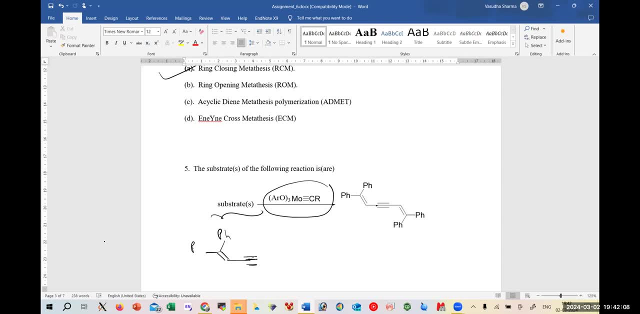 something like this way, or it is, having the substrate could be possibly be R this one. So here, this is the only option if I am taking these two same groups. that is self metathesis. So the star marks will give you one product and this CH3, alkyne CH3 would leave as another product. 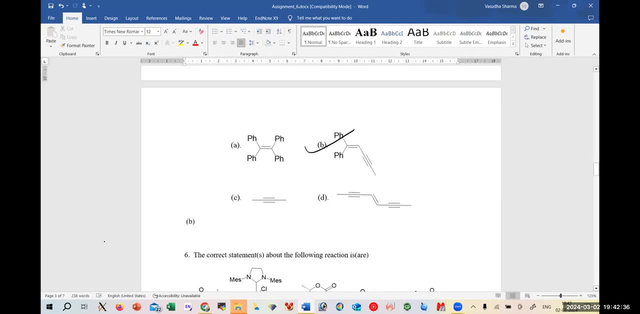 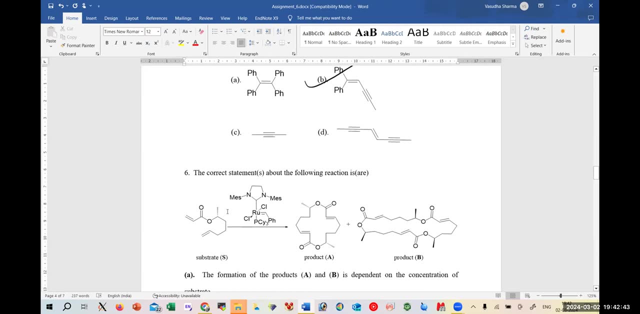 So therefore the fifth, for question number fifth, the answer is B. Now the correct statement about the falling reaction. We have here alkyne groups in presence of the metathesis. Now it is giving you a dimer and a trimer. 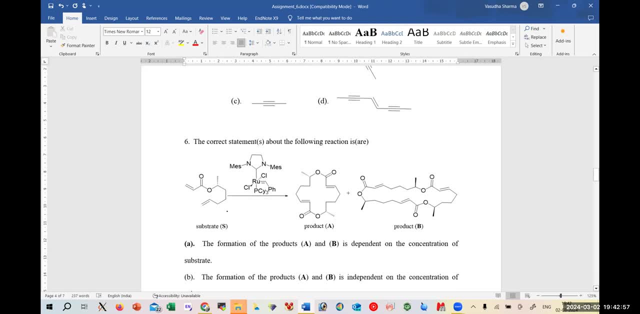 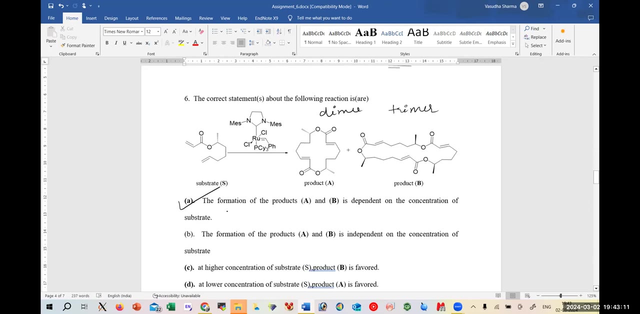 So this is the tandem ring closing metathesis. Now we already know dimer and trimer. concentration is dependent on the concentration of the substrate. So yes, A option is right And if it is independent, no, it's wrong. At higher concentration the product B, the trimer, would be the major product. 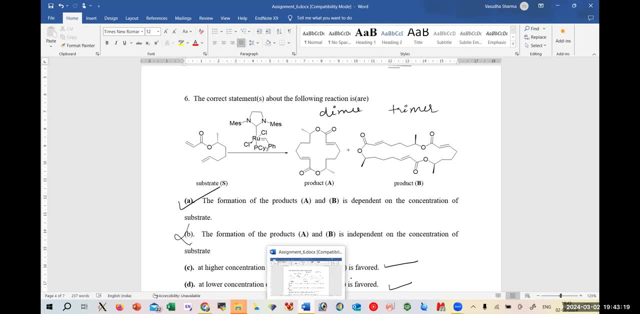 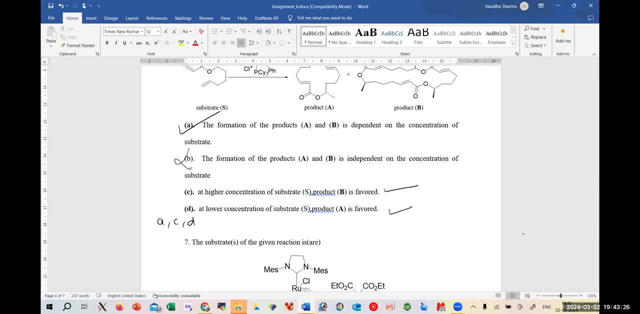 Yes, if, at lower concentration, product A would be the major product, which is absolutely right. So these are the three options which are right, which is A, C and D. These are the right options. Now we have the seventh question: as the substrate of the given reaction. 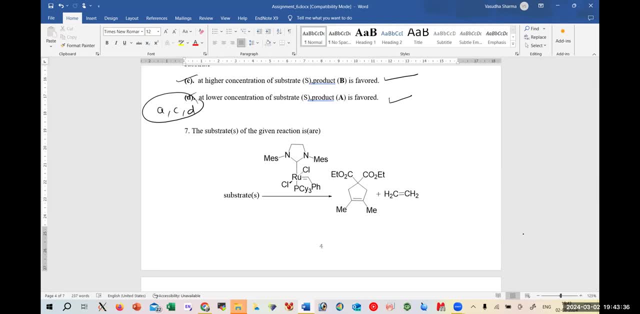 So here, if you'll see again, this is a metal carving And we are having a closed ring with a cyclic with an ethylene molecule out. So this could only be possible if we are having a substrate kind of this way which is having here neath side and here it is having 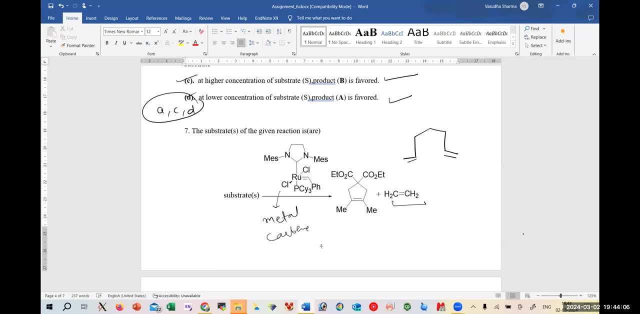 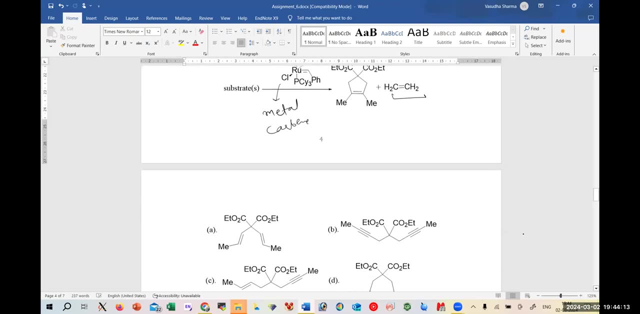 There is methyl and there is double bond, And there only you could form. So the option B is your right option, where it is having this particular product, Where these two combine and therefore it would form here. If this is the case, these two have to combine, which is not possible. 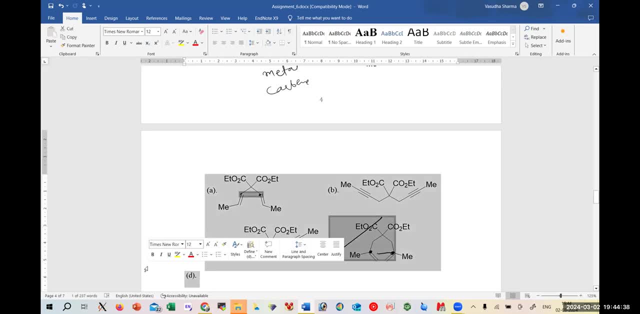 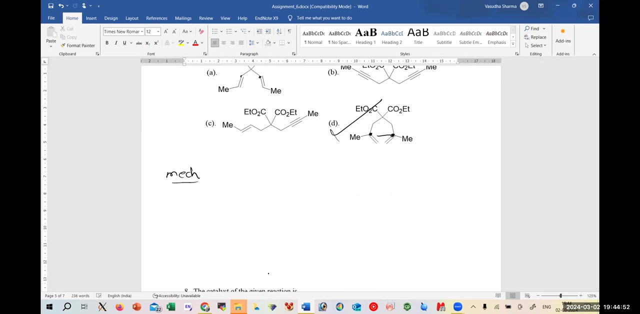 So the option D is the right option. What is actually happening here If I'm taking Methyl C02. Et. So this dotted and this star mark. So this would be one, two, three, four and five. We'll quickly make the five moment ring with a double bond. 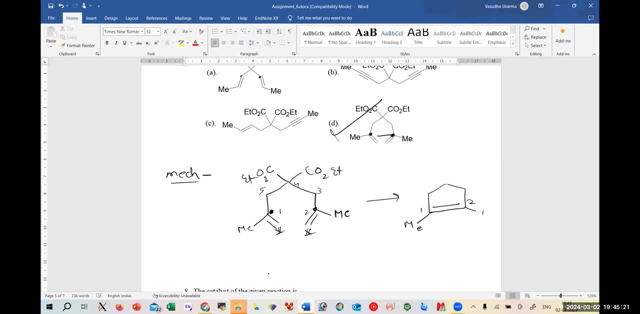 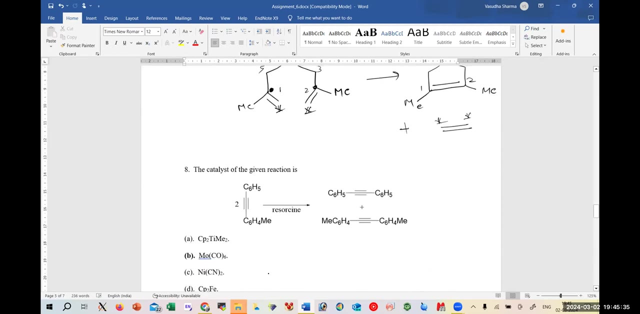 And here one was having and one and two are having methyl substituents. Four is having C02 et substituents Plus star. It's nothing but the ethylene molecule. So this was been asked and the question seven is done. Now we have the catalyst of the given reaction. 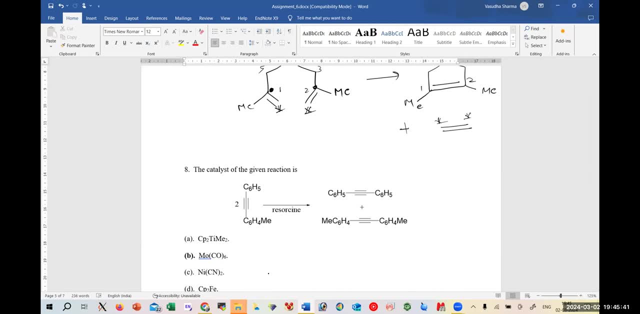 Here again, if you see C6H5.. They are combining together to give you this product If I'm taking this molecule, This also. we have discussed C6H4Me, C6H4Me, So they both will combine together. 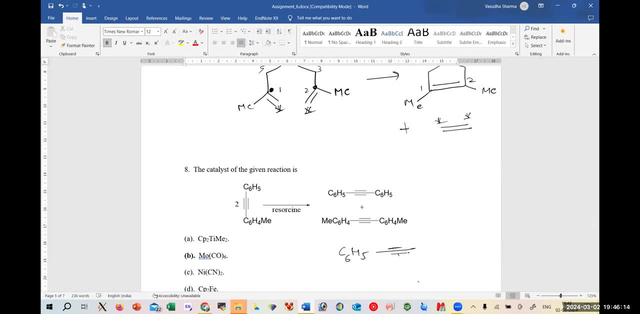 So if they are having C6H5.. Triple bond, C6H4Me And similarly on this side, also the two units we are taking, So they would give you a self metathesis product Which is C6H5.. C6H5. 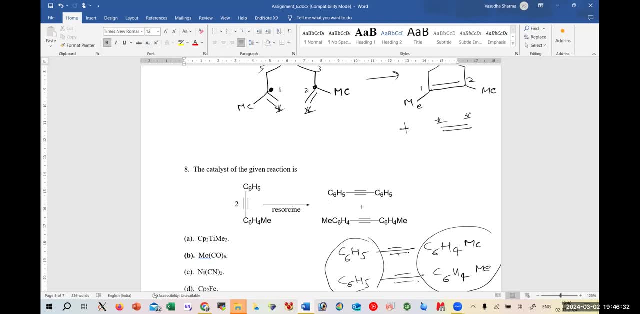 And C6H4Me And in presence of what catalyst is happening. So we have already seen it happens in presence of molybdenum catalyst And resource seen in 160 degree Celsius. So it's an alkyne metathesis. 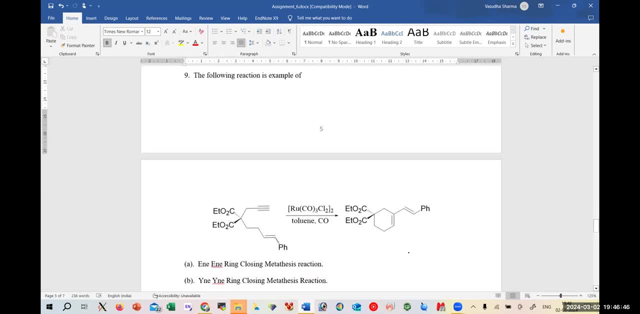 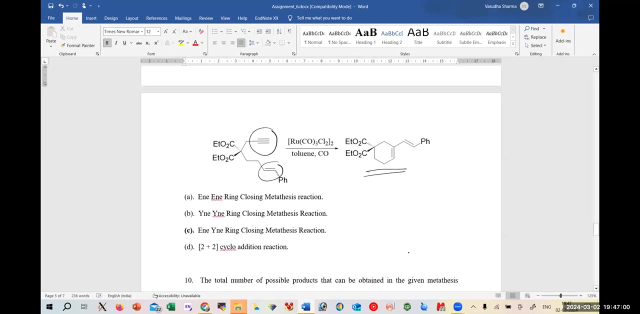 Now the ninth question says the following: reaction is an example. Now here, if you will see, We have an alkyne and ene And we can see the closing of the ring And it is having the alkyne over here. It is nothing but your ene mechanism. 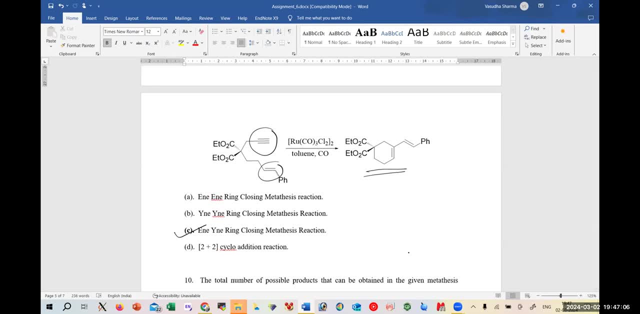 Because only then it is possible to have this kind of molybdenum Where 1,, 2,, 3,, 4,, 5 and 6.. So this is your 1,, 2,, 3,, 4,, 5 and 6.. 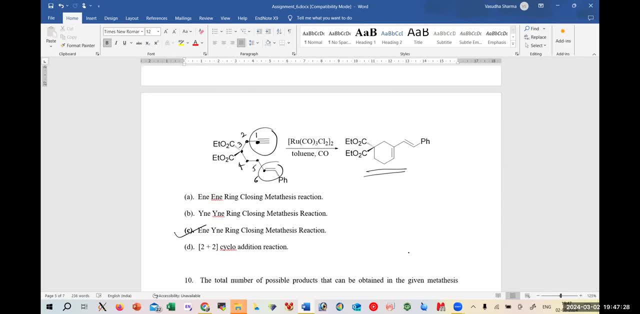 Which is what 3,, 2,, 1, 5.. to the actual things undergo with respect to the mechanism where the metal carbine would undergo with the two alkenes, would one alkenes would undergo the metal carbine and then 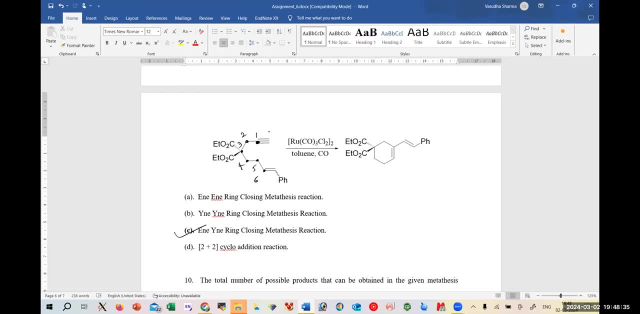 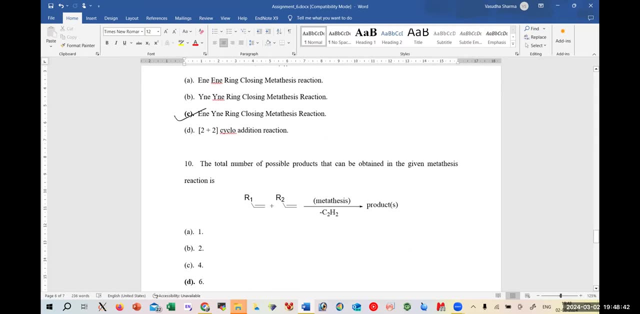 subsequent. subsequently it would undergo the alkane metathesis. so this is in iron ring closing metathesis reaction and the last is the total number of possible products that can be obtained in this metathesis reaction. so we have R1. since it is, it can be possible. 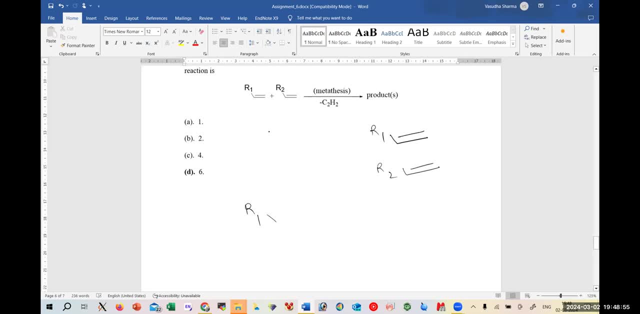 to give you R1 and R2 and also be giving you R1 and R1 and R2 so both can be having a. obviously, CH2 is not available, R1 isn't available, there is none installed. so, Irene, as you can see, we continue between. 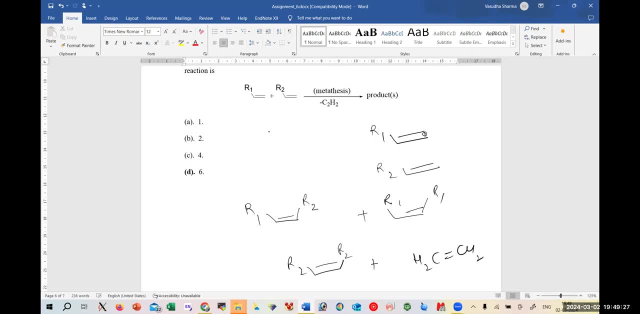 R2 and R21ine and R, three radii, like I was. comments. like I said5 goodness, you want me to read the Chinese maritime expresseddrags. yeah, whether or not, what you like to feel about R3 and therees another one, CH2, would be there in every part where one part is going to connect with other one, since 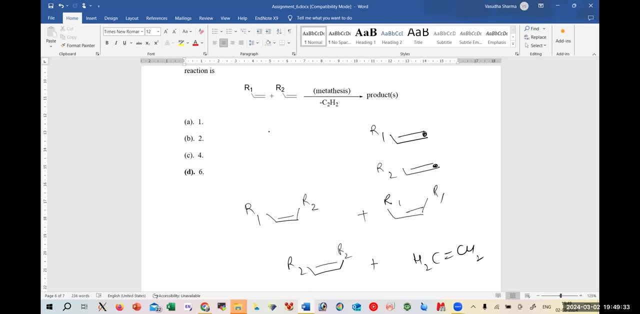 we will be having three different possibilities. these two combine or two molecules of this, one combines with this one, or R2 combines with R21.. So these are three possibilities which could give you one product, second product third, and three molecules of this CH2CH2..